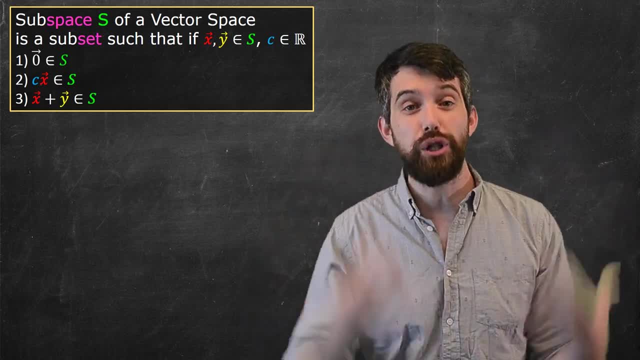 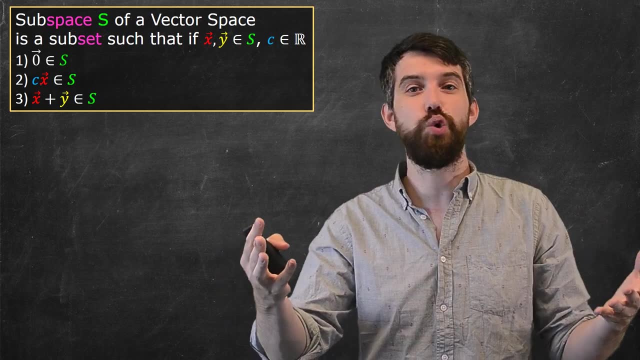 English for the last two properties is that our subspace is closed under scalar multiplication and closed under vector addition, Which just means that you can do as many scalar multiplications as you want, as many vector additions as you want, and you remain in the subspace. 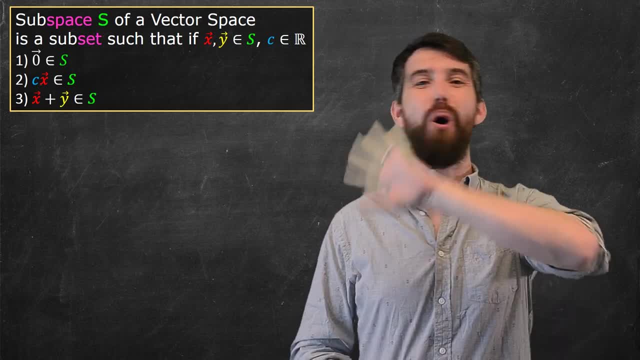 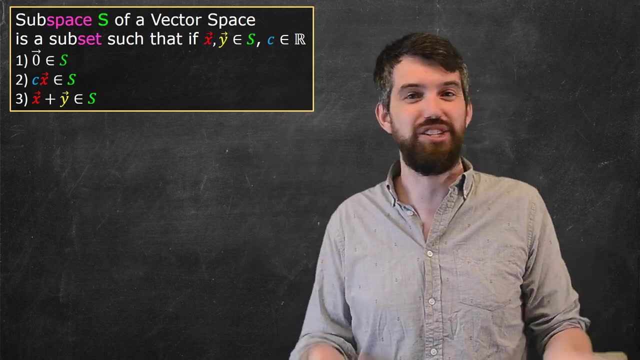 Okay, so that's our definition and I like this because now all the linear algebra we were doing, we can do it on a subspace, because all of linear algebra is basically just doing scalar multiplication and vector addition. So subspaces are basically the subsets where you can do linear algebra. 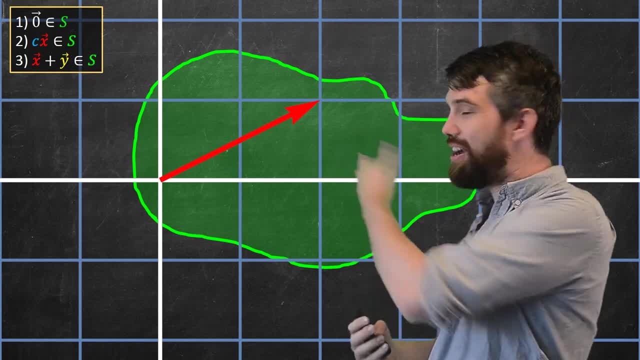 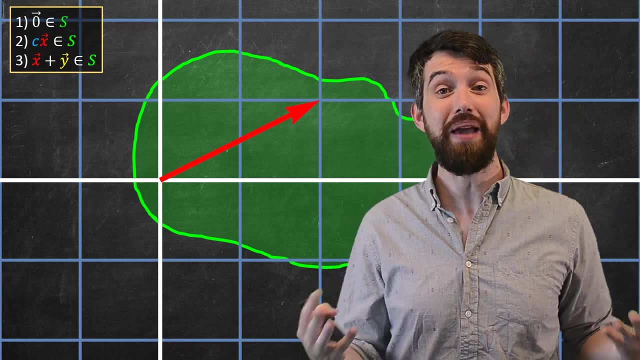 Okay, let's see a few different examples. Okay, so I've got some vector here. It is living inside of this green subset. Now the question is: is this subset a subspace, As in? does it obey our three different properties? Well, let's see. First of all, 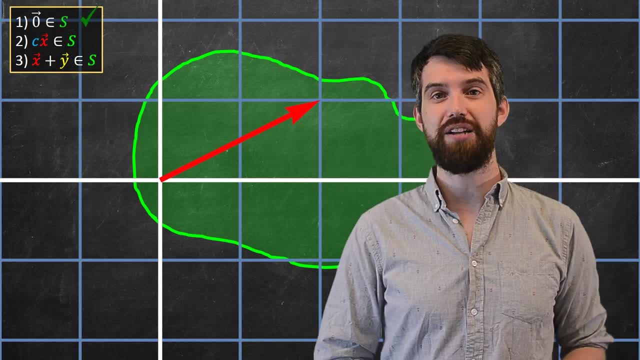 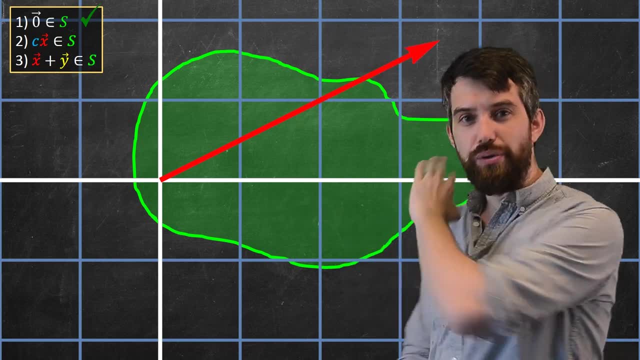 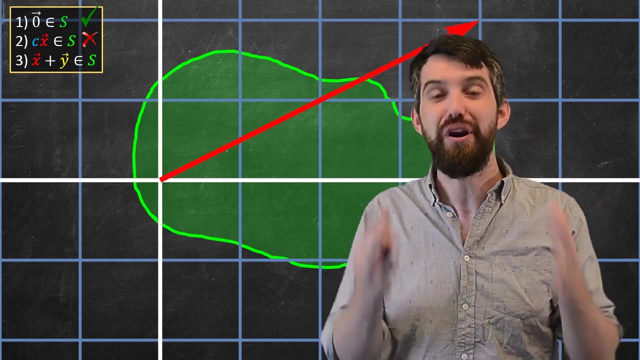 the zero vector does indeed live in this thing. We have this zero vector. So, yes, first property is checked. Second property: Okay, I have this red vector. Let's multiply it by two, Let's do a scalar multiplication. But now my vector has left the subset and so I don't have the second property and therefore, 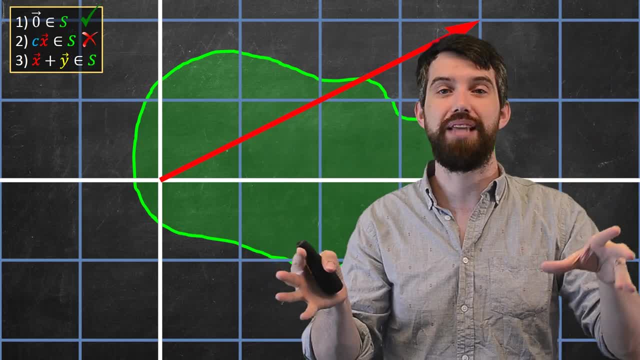 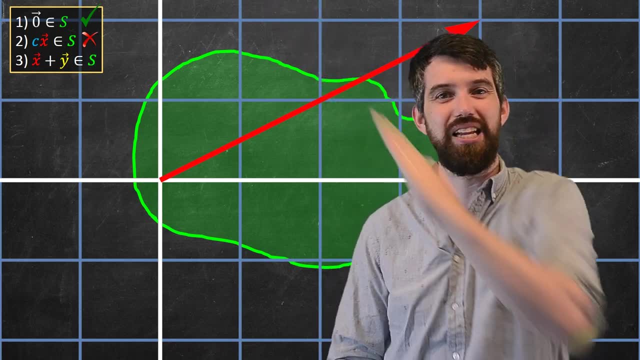 this is not a subspace. This sort of random blob I put down is a subset but not a subspace. And in fact there's sort of a lesson here, which is that if I've got one vector and scaling it to sort of 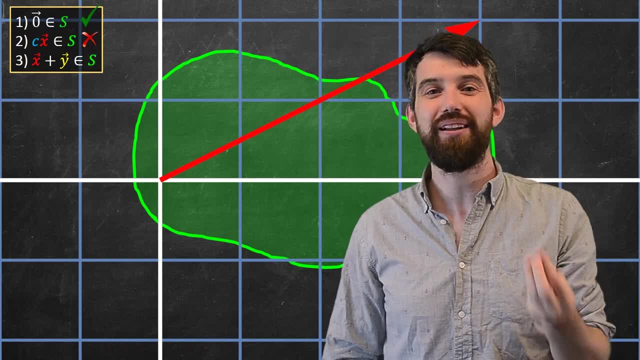 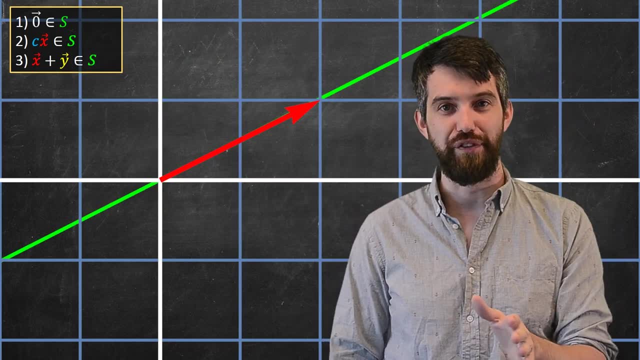 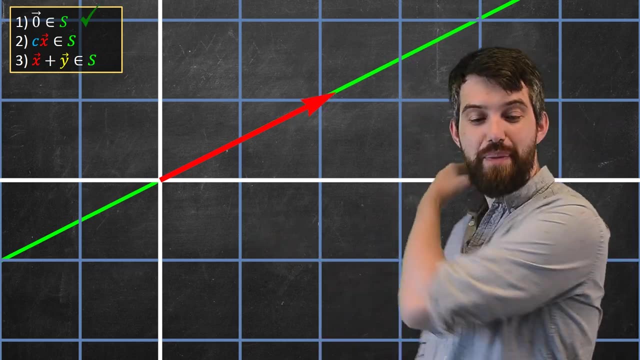 send stuff along a line. probably I need to have at the very least infinite lines if I'm going to be talking about subspaces. So let's see that example. Okay, I have my infinite line here, Wonderful. So zero vectors on that. That works If I take this vector and I say, multiply it by a factor of two. 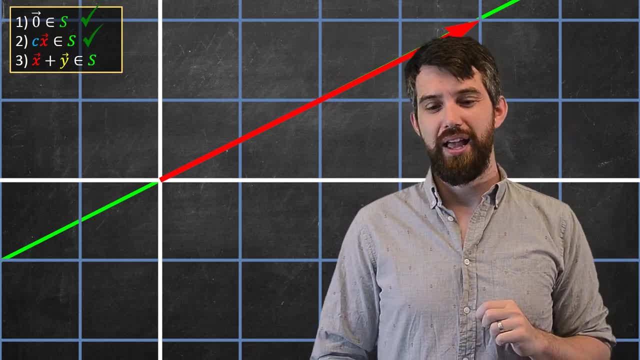 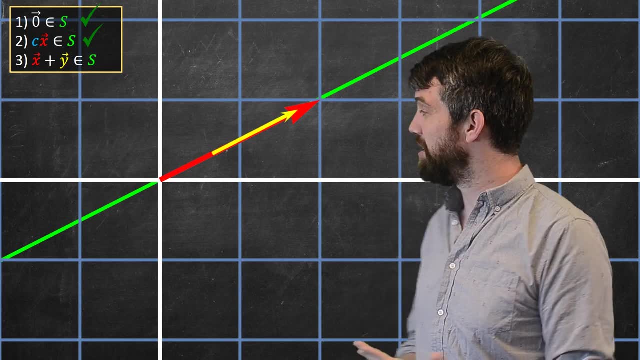 it's still on the line. So, yep, that one works as well. And then if I take the red vector but I add some other vector, some sort of yellow vector, to this, well, how do I add these in the tip-to-tail manner? 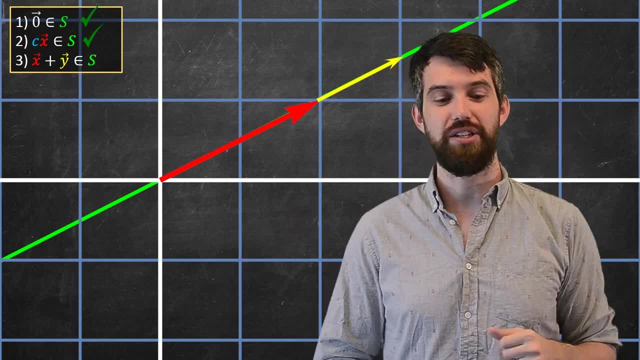 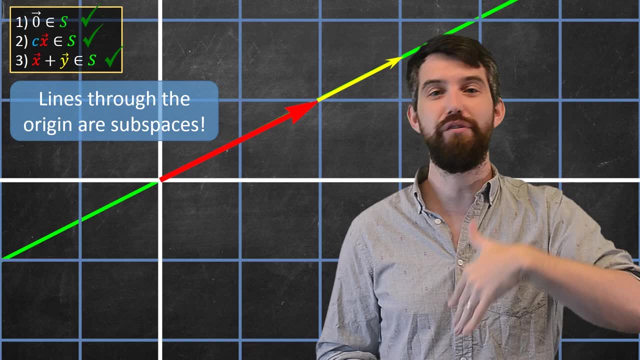 So I line them up, the red, then the yellow, and I'm still on the line. So all three of my properties are indeed true and therefore lines through the origin are going to be subspaces. You can move this line wherever you want, but it has to go through the origin. 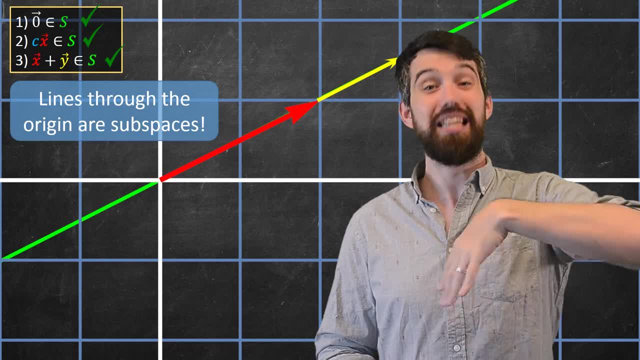 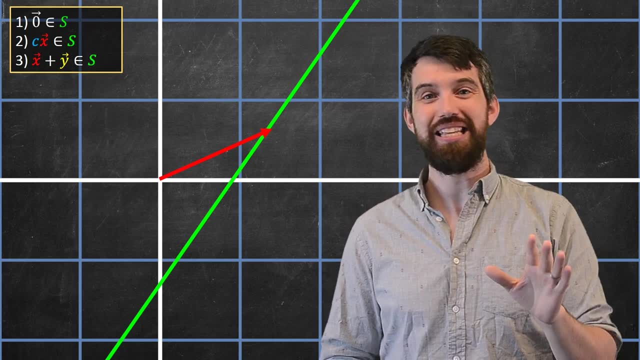 Well, does it have to go through the origin? Let's try that, Let's okay. let's now look at a line that does not go through the origin. So here's an example. Now you might just say: look, Trevor, this is actually really easy. The zero vector's not a line. 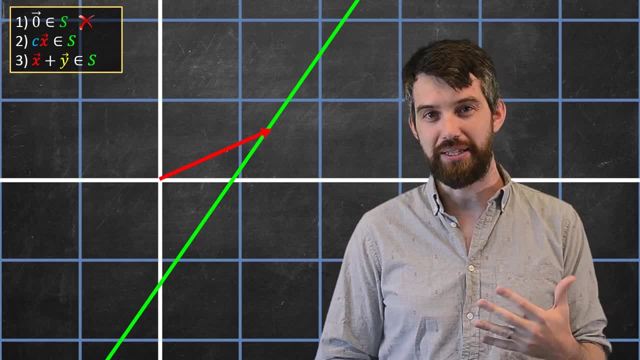 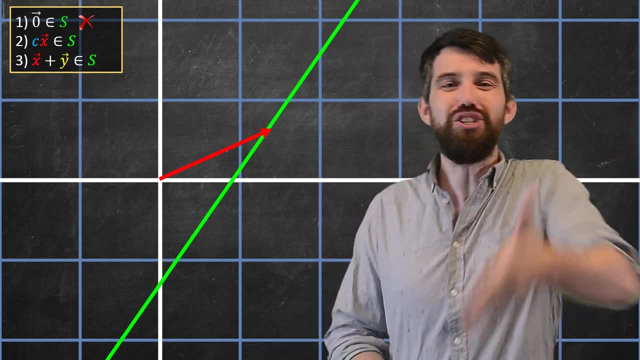 so clearly. this is not the origin, It's not going to be a subspace. Then you might ask: well, hold on, why are you even asking? why are you demanding that the zero vector's on here? So let me show you some of the reasons why this fails. Okay, we've got this one vector on it. 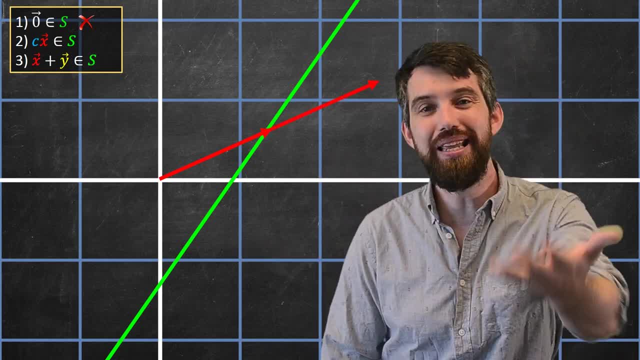 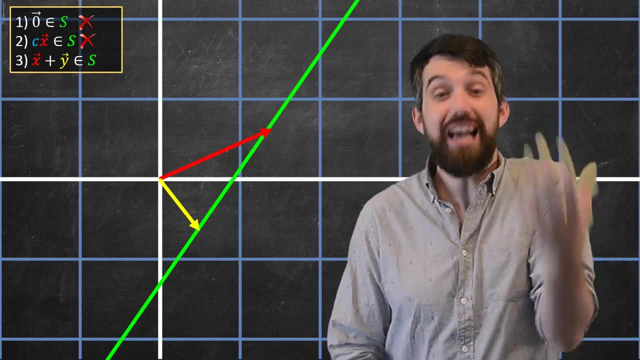 What about if I multiply it by two? if I stretch this out, Well then it immediately leaves. So, indeed, the second property is also false. All right, what if I take one vector on the line and a second vector on the line? 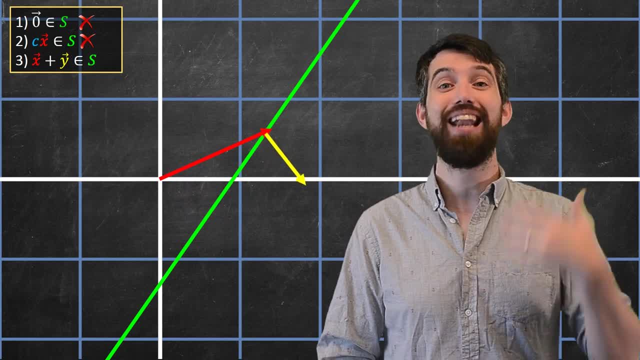 Well, okay, if I want to add them, I have to add them up in my tip-to-tail way, and again I get off the line, And so my third property is false. So a line not to the origin is really not to the origin. 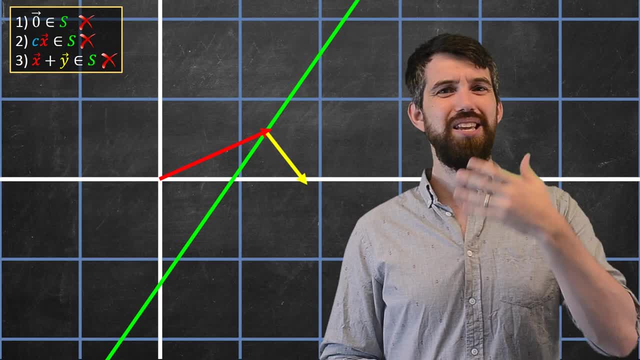 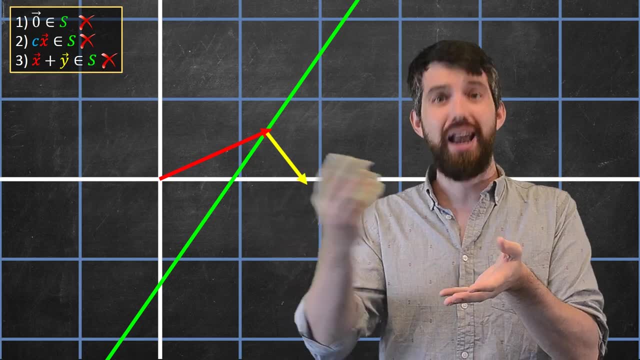 It wasn't just this first property that violated it. In fact. what is the role of the first property? anyways, If you look at the second property, if I've got any vector, I can multiply it by zero and I get the zero vector. 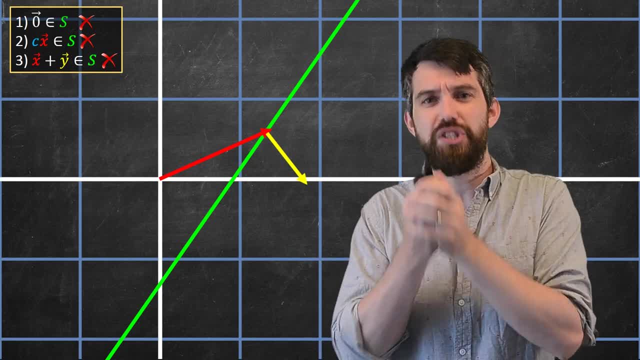 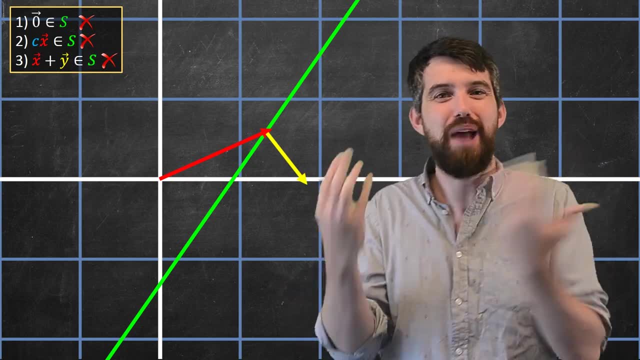 So, in fact, any subspace is always going to have the zero vector by the second property, except one: It's the empty set. The empty set where you don't have anything to begin with, and so you can't multiply by zero. 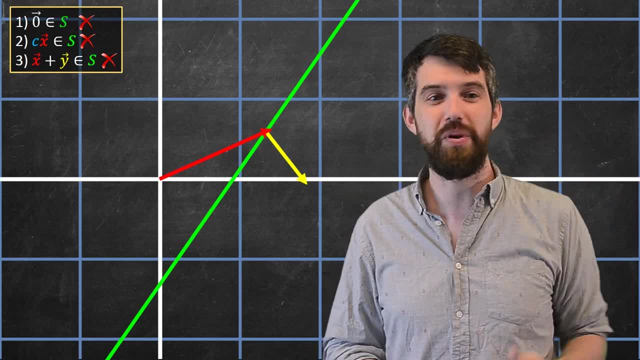 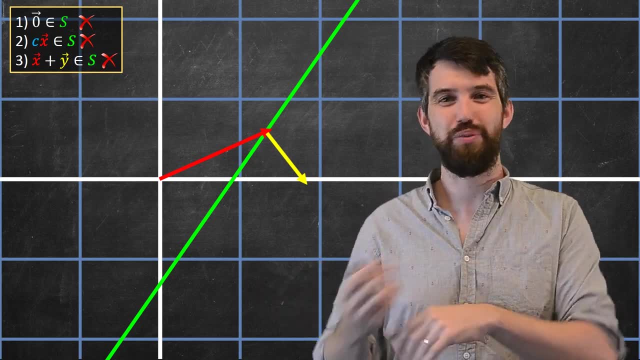 So really, the only role of the first property that says zero has to be in there is to get rid of the sort of boring, trivial case of the empty set. Indeed, a lot of our theorems are going to be a little bit nicer in the future. 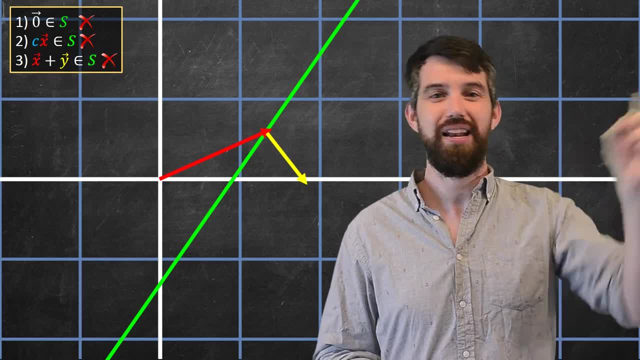 which you don't ever have to worry about. the empty set. so we're just going to put that right there in our definition. You need to have the zero vector in it, even though it's kind of a consequence in every case, but the empty set. 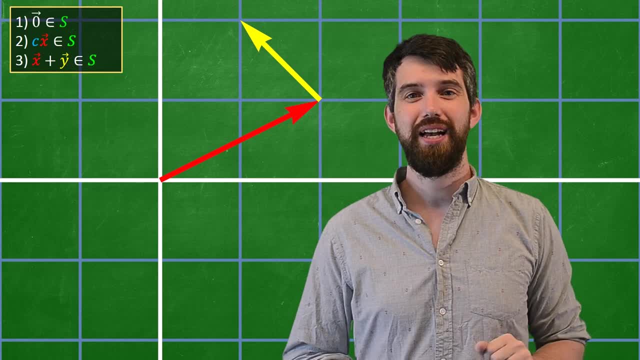 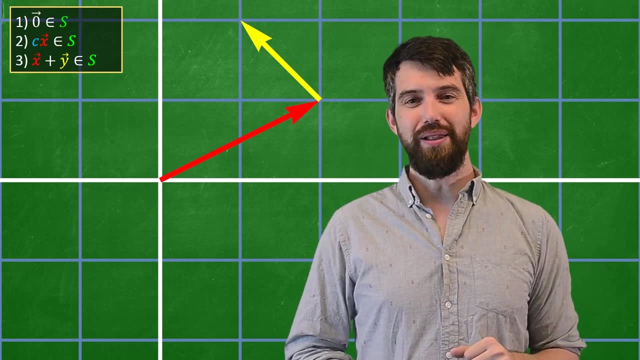 Two more slightly pathological examples, but they're important ones. This one is everything, All of Rn, or in this case, R2.. So I just sort of shaded everything green. Well, this, almost trivially, is going to be a subspace. 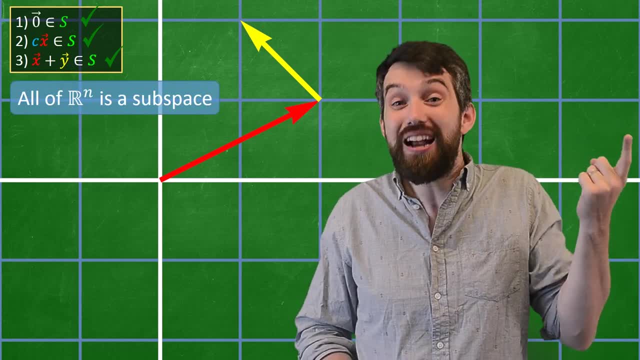 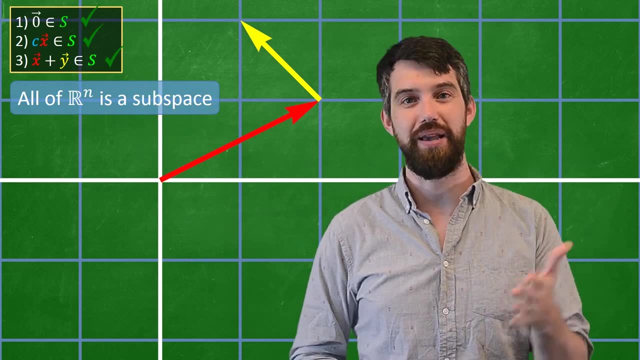 I've got the zero vector because it's got everything. If I add any pair of vectors, they're going to clearly just be in there. They can't leave it. If I stretch them, they can't leave it. So this is going to be a subspace. 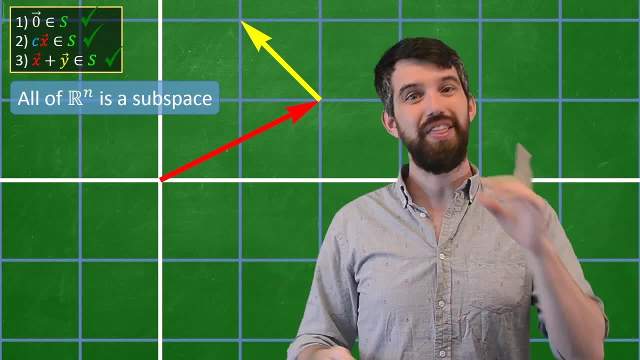 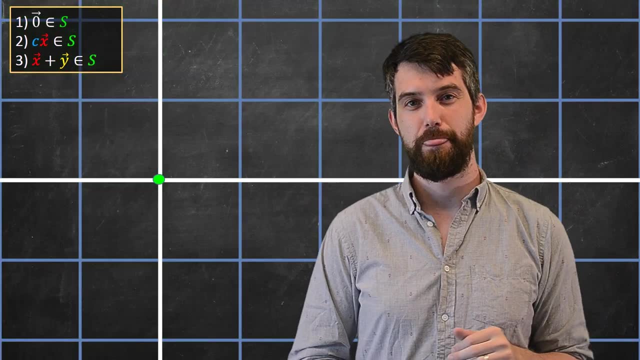 It's that sort of trivial subspace, the subspace that's everything. The other trivial one is the one that's the smallest possible one, It's just zero, And I know there's a green dot there, right at zero. Well, the zero vector's on there. If I take the zero vector, I multiply it by two.